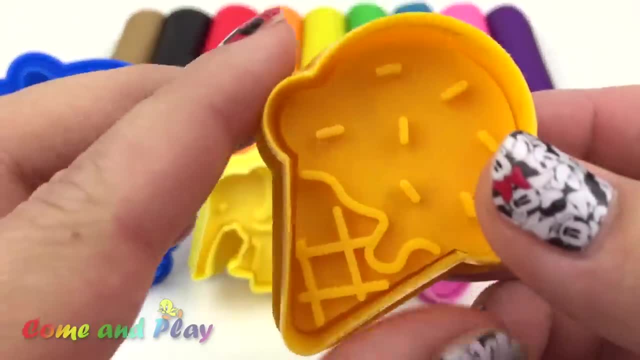 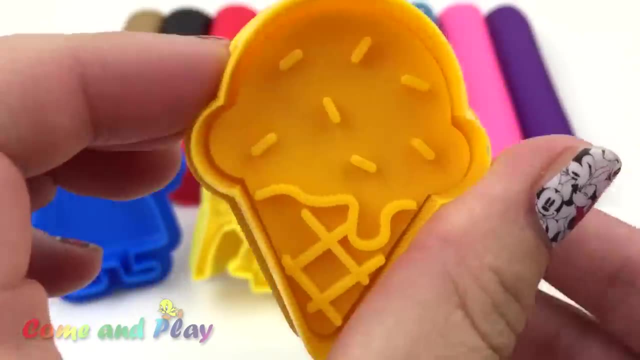 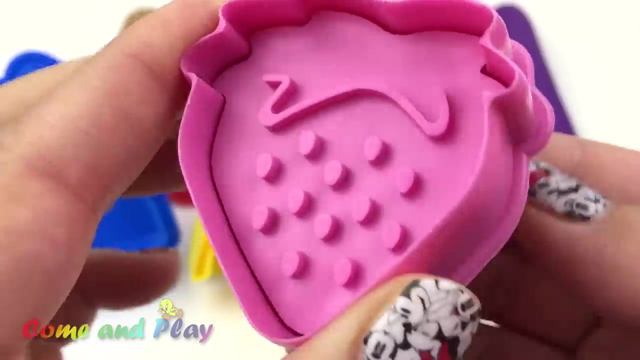 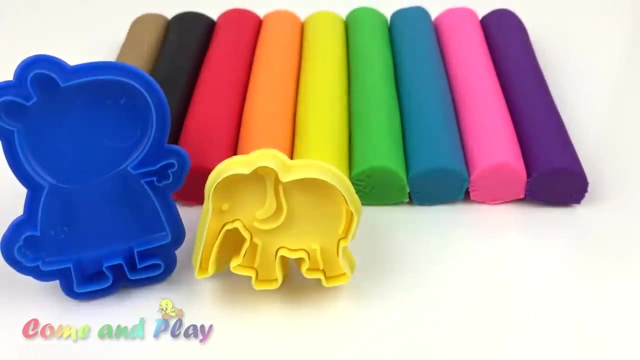 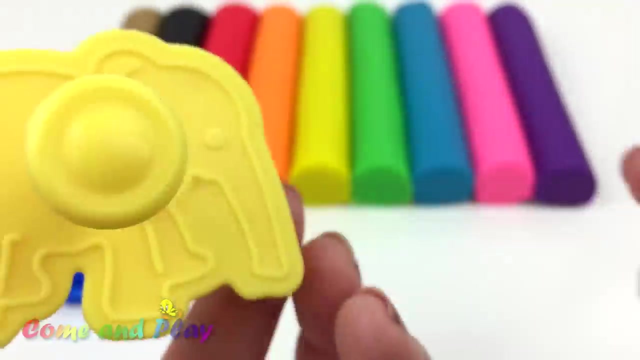 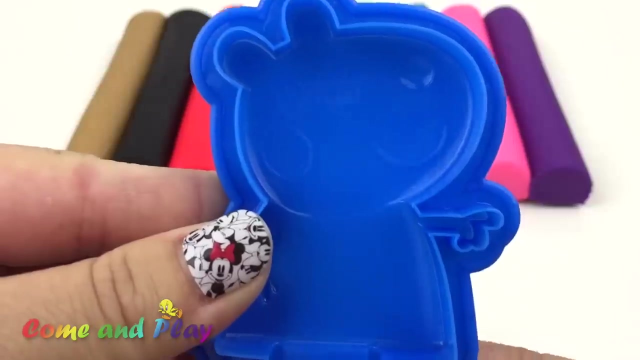 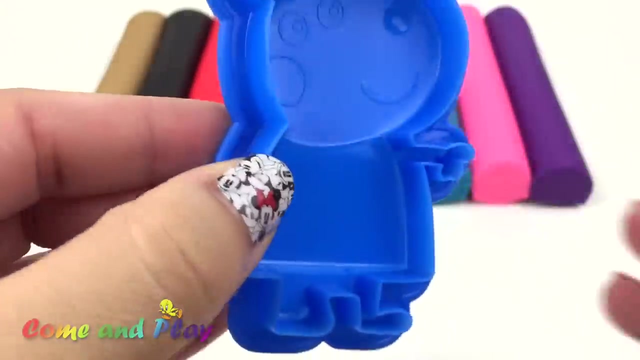 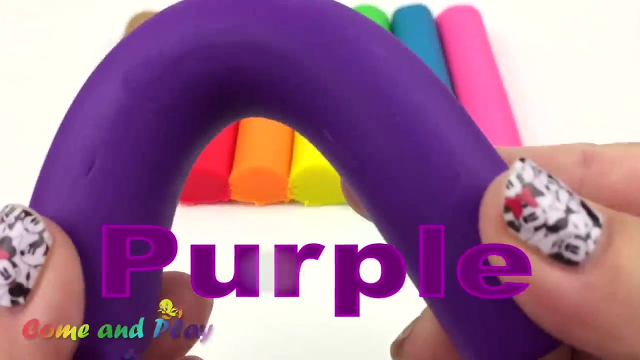 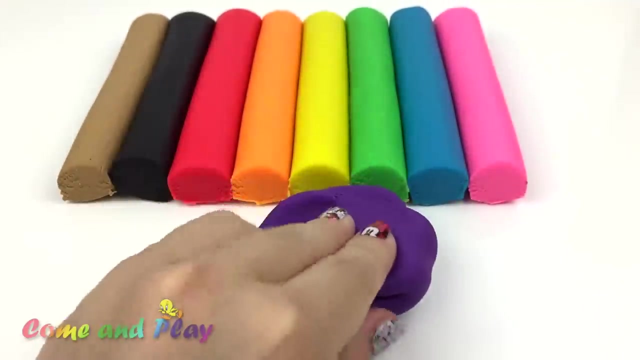 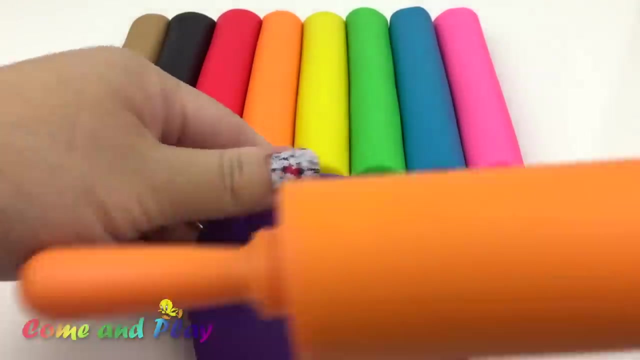 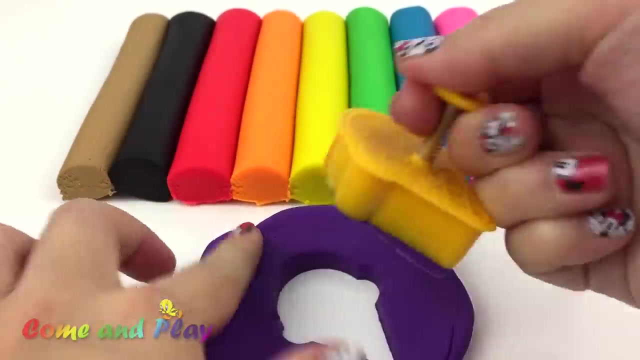 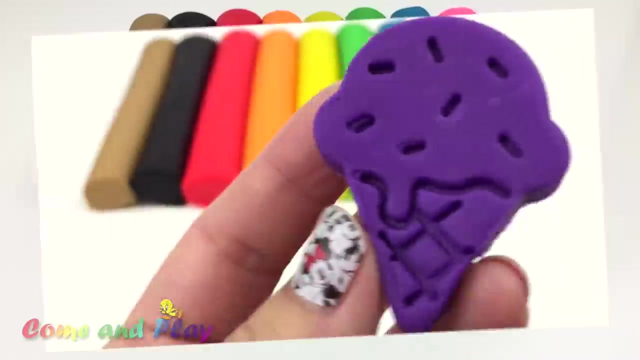 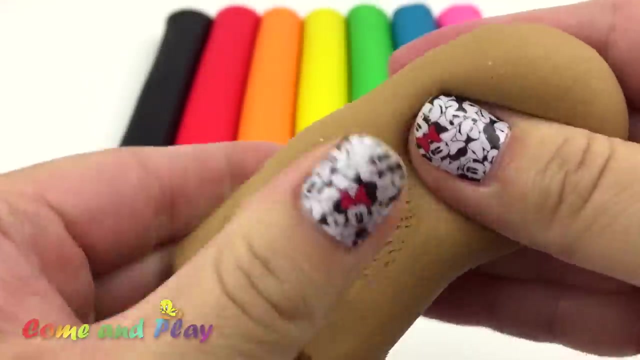 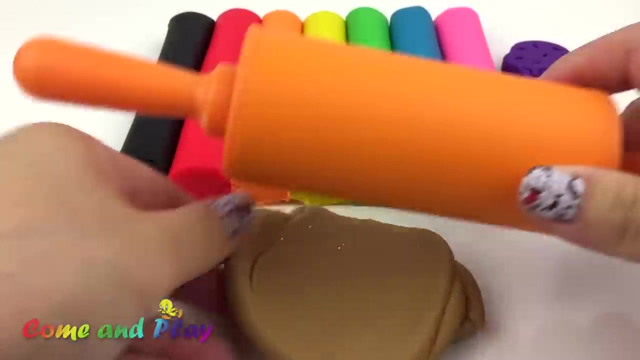 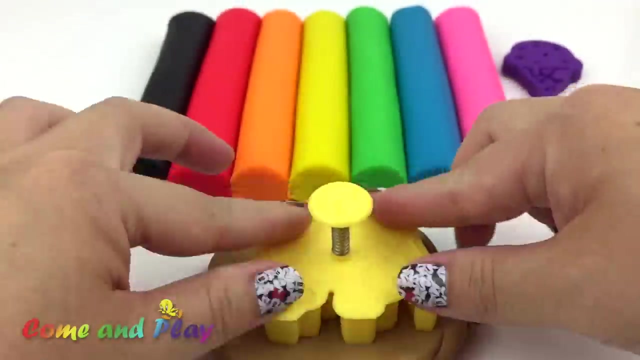 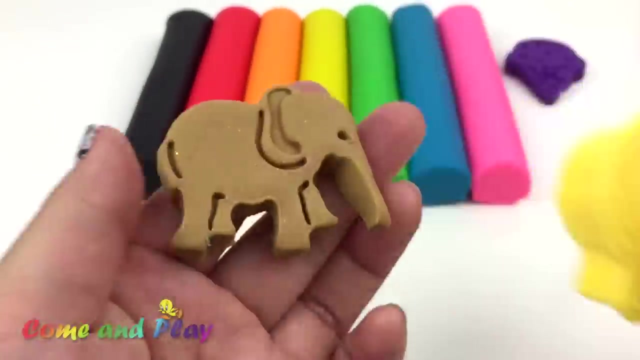 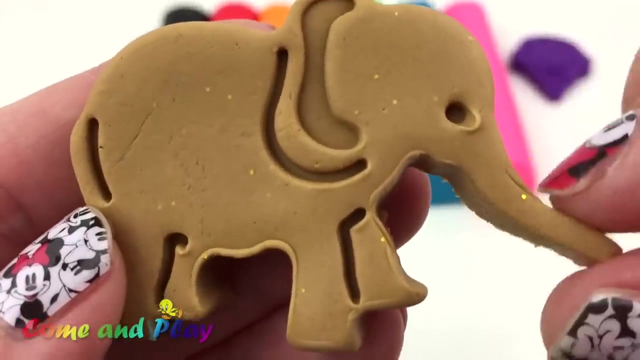 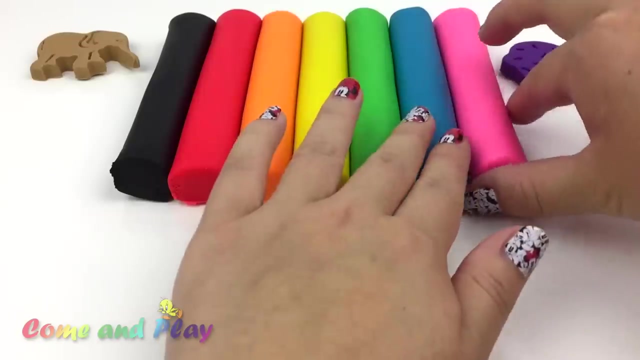 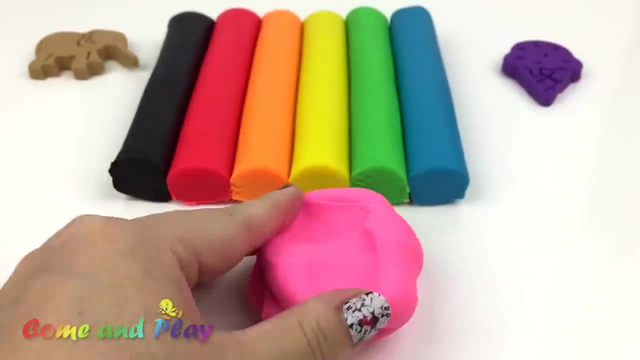 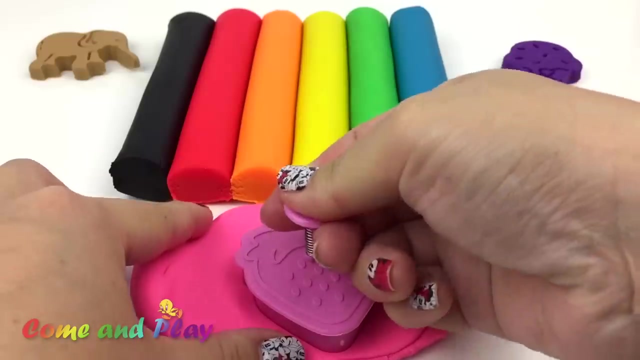 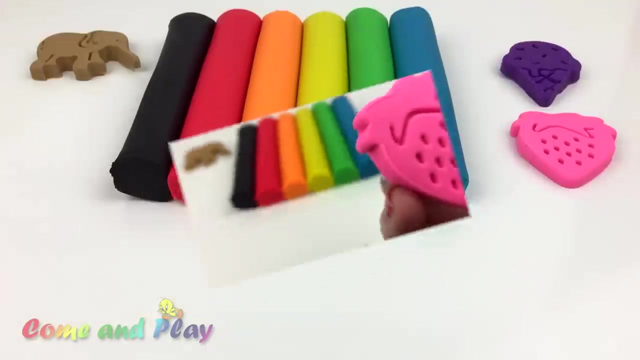 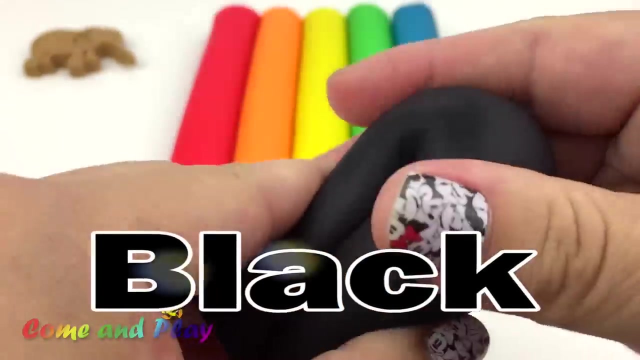 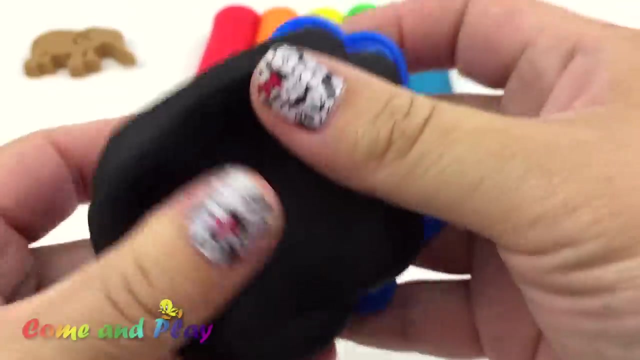 Thank you for watching. Purple, Brown, Yellow, Green, Yellow, Blue, Yellow, Red, Yellow, Blue, Yellow, Blue, Blue, Yellow, Blue, Yellow, Blue, Blue, Pink, Yellow, Yellow, Blue, Pink, Pink, Pink, Purple, Yellow, Yellow, Blue, Blue. A tisket, a tasket, a green and yellow basket. I wrote a letter to my love and on the way I dropped it, I dropped it, I dropped it. and on the way I dropped it, A little boy. he picked it up and put it in his pocket. 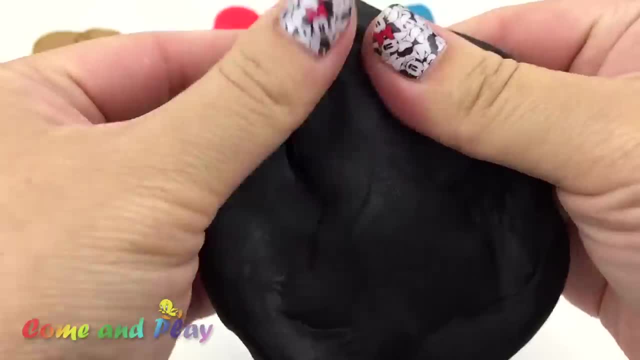 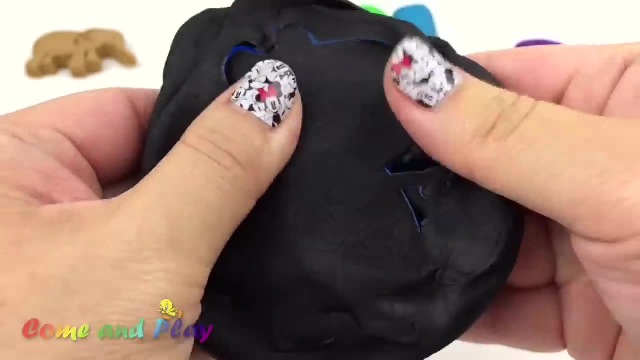 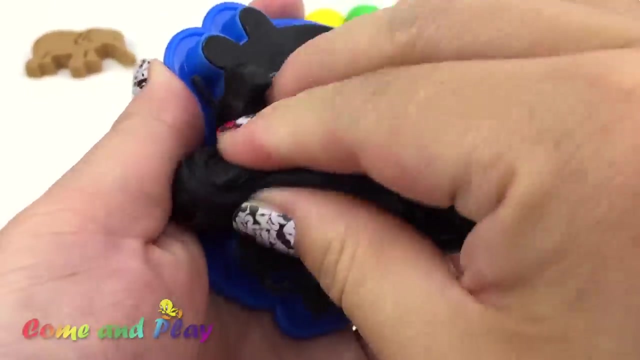 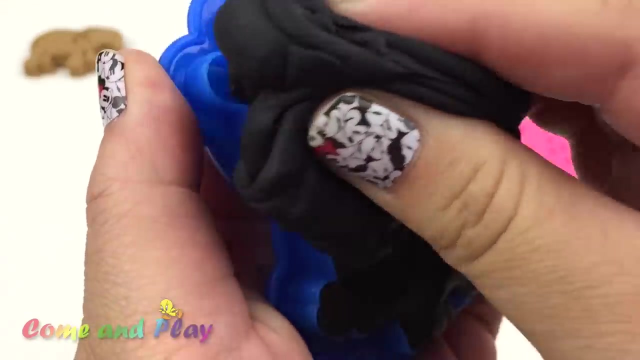 A tisket, a tasket, a green and yellow basket. I wrote a letter to my love. and on the way I dropped it, I dropped it, I dropped it. and on the way I dropped it, A little boy. he picked it up and put it in his pocket. 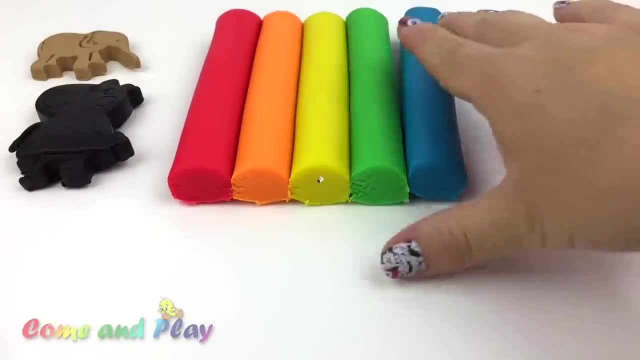 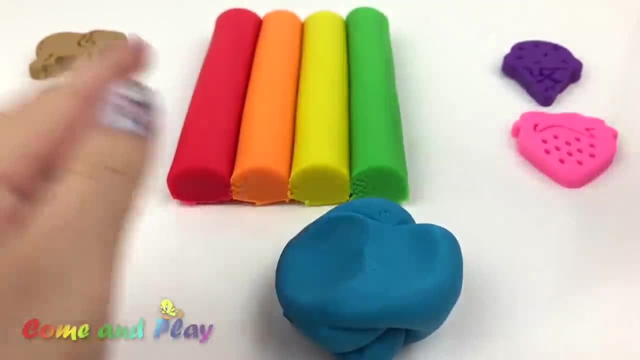 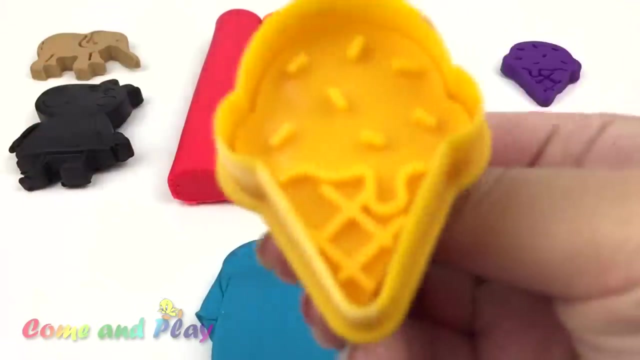 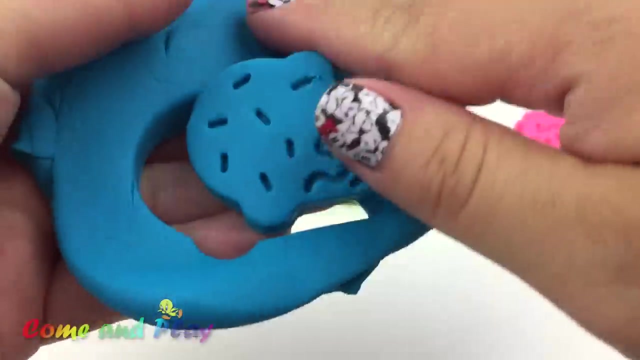 A tisket, a tasket, a green and yellow basket. I wrote a letter to my love and on the way I dropped it: A tisket, a tasket, a green and yellow basket. I wrote a letter to my love and on the way I dropped it. 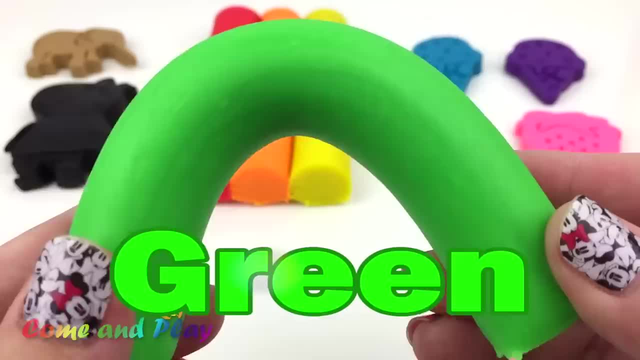 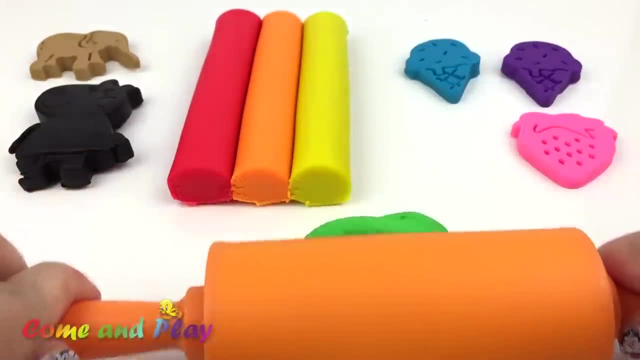 A tisket, a tasket, a green and yellow basket. I wrote a letter to my love. and on the way I dropped it, I dropped it, I dropped it. and on the way I dropped it, A little boy. he picked it up and put it in his pocket. 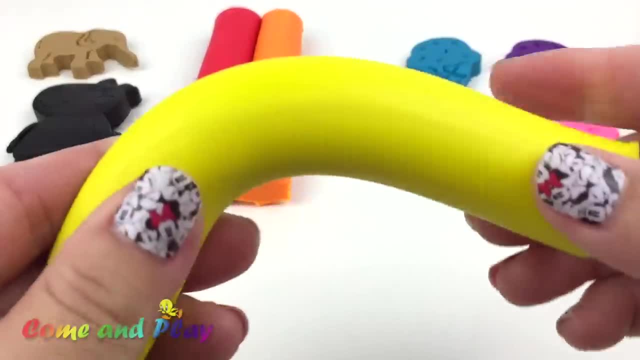 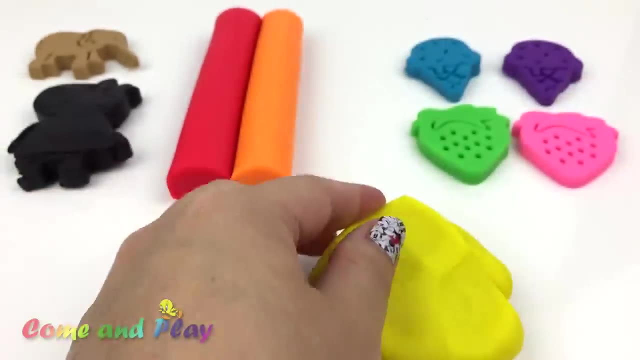 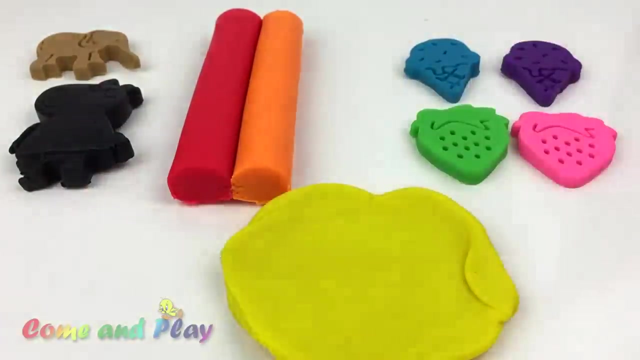 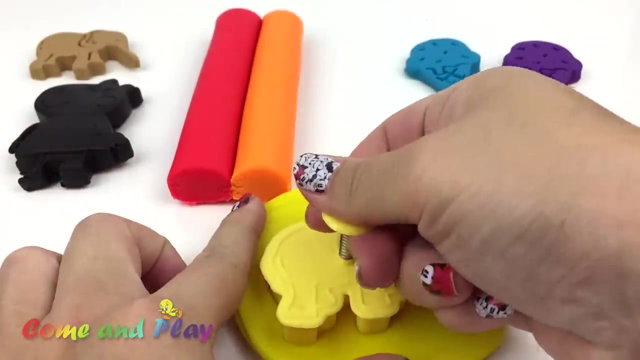 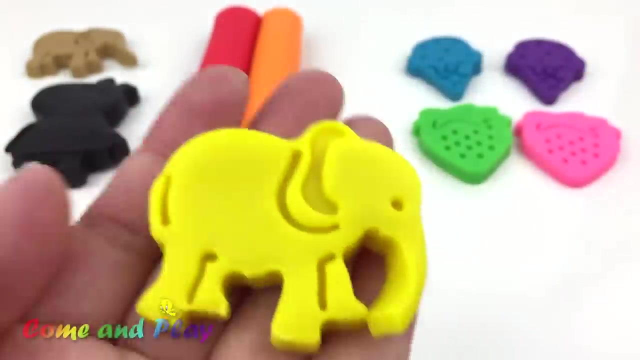 A little boy. he picked it up and put it in his pocket On the way I dropped it. put it in his pocket On the way I dropped it. On the way I dropped it, I didn't mean it, but it. 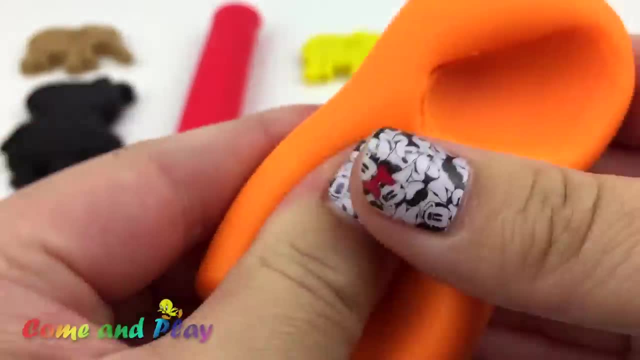 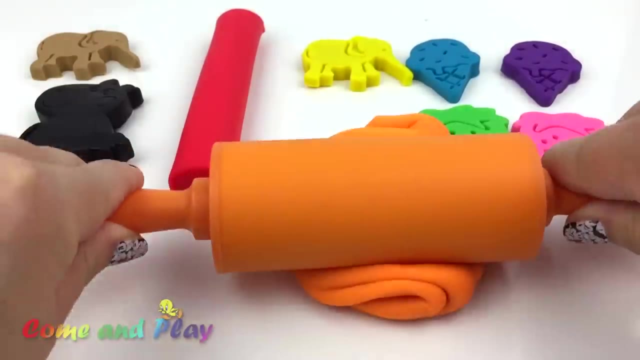 Orange Lou Lou. skip to my Lou Lou Lou, skip to my Lou Lou Lou. skip to my Lou, Skip to my Lou. my darling Flies in the buttermilk: shoo, fly, shoo. 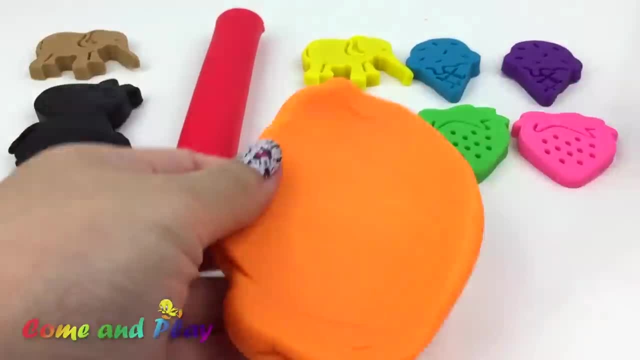 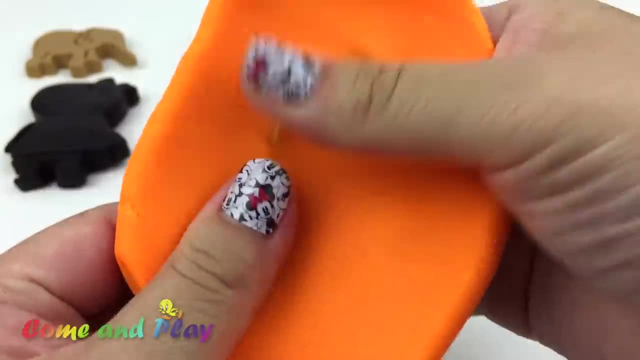 Flies in the buttermilk. shoo fly, shoo. Flies in the buttermilk shoo fly, shoo. Skip to my Lou, my darling Lou Lou. skip to my Lou. Lou Lou, skip to my Lou. 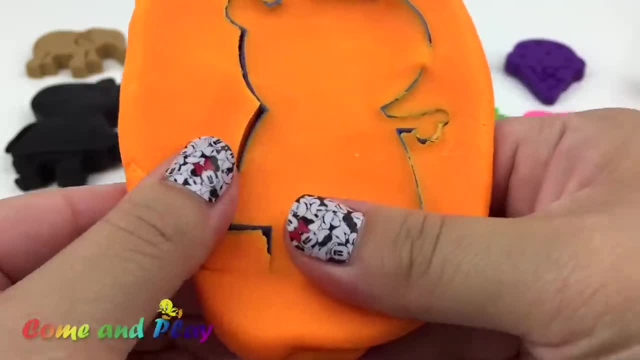 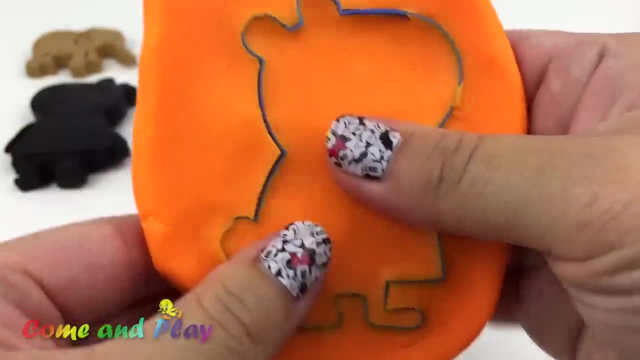 Lou Lou. skip to my Lou. Skip to my Lou. my darling Cats in the cream jar, ooh ooh, ooh. Cats in the cream jar, ooh, ooh, ooh. Cats in the cream jar, ooh, ooh, ooh. 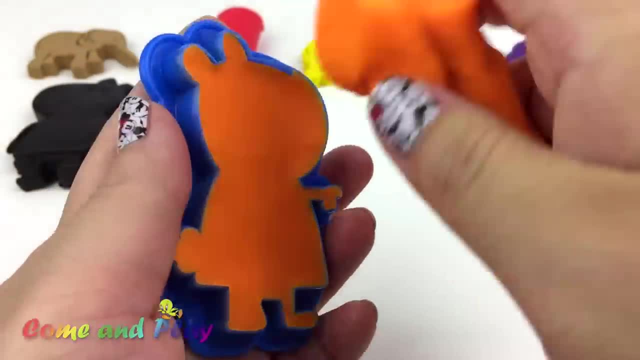 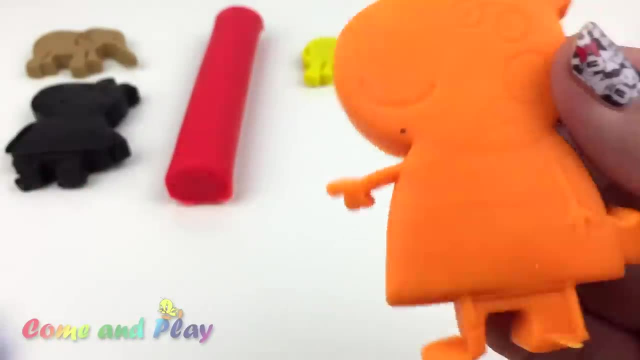 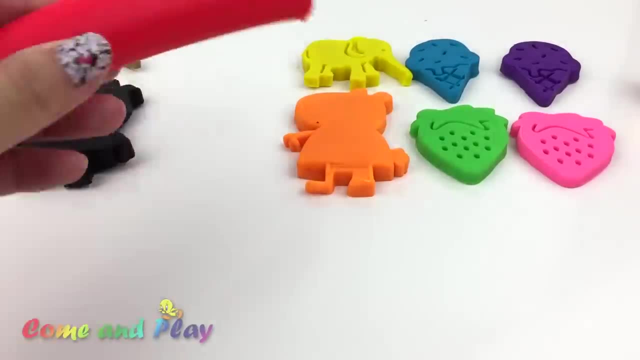 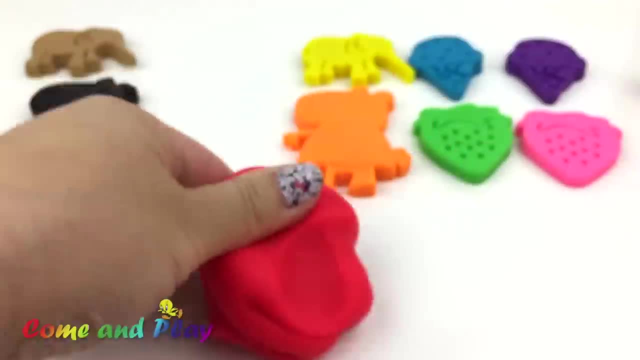 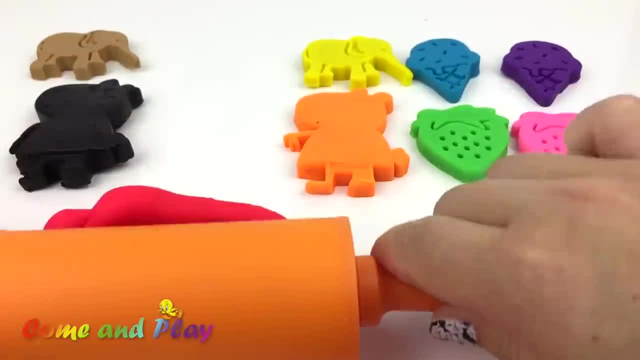 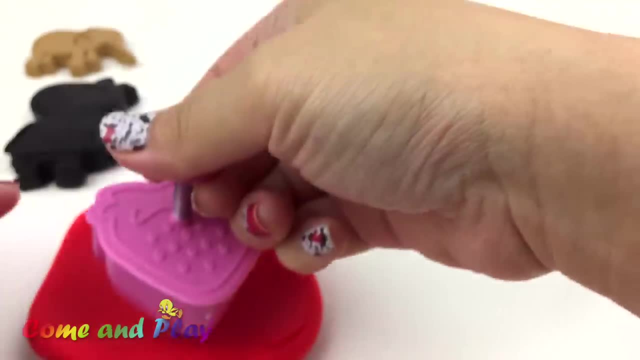 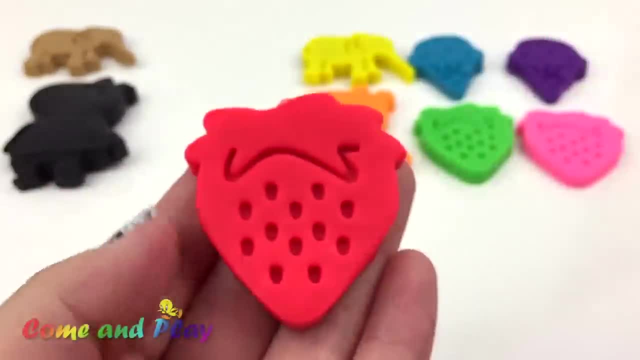 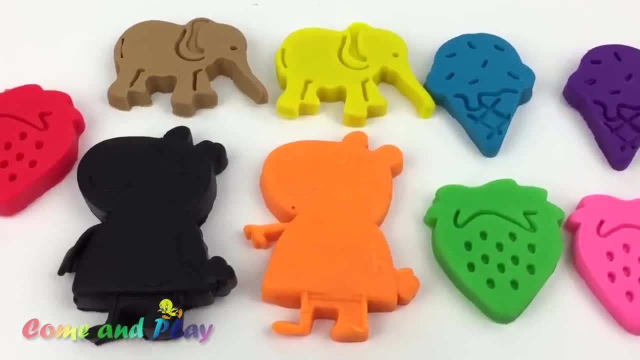 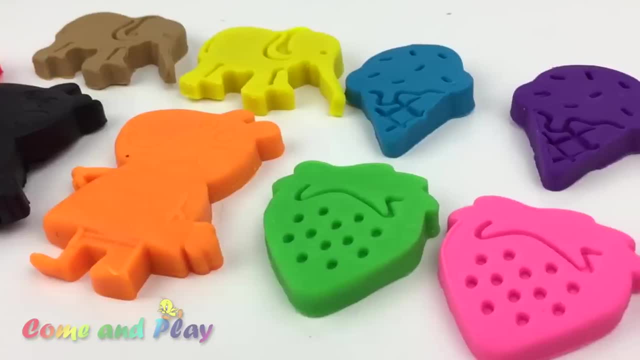 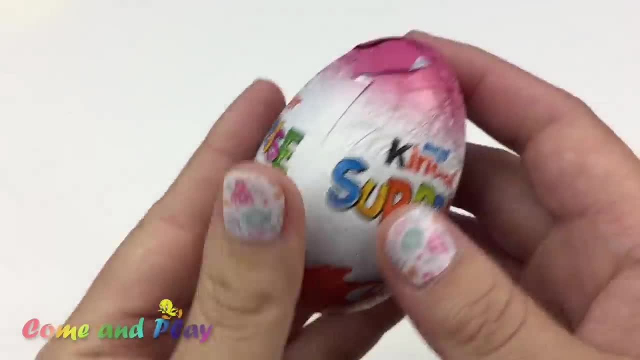 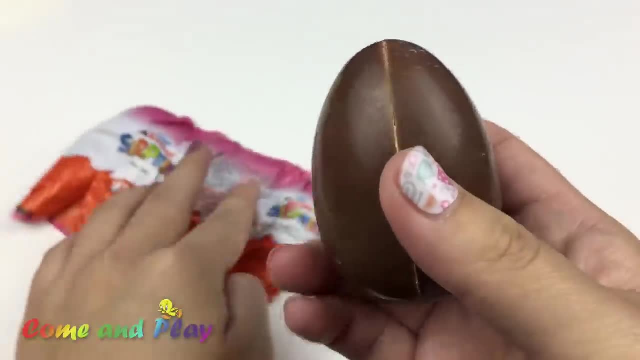 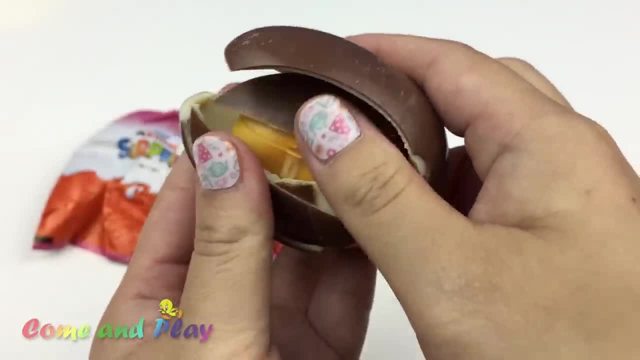 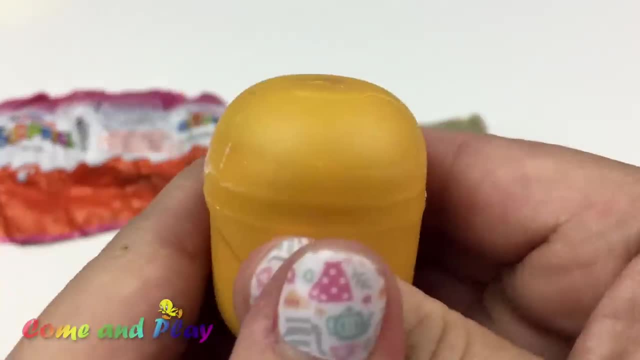 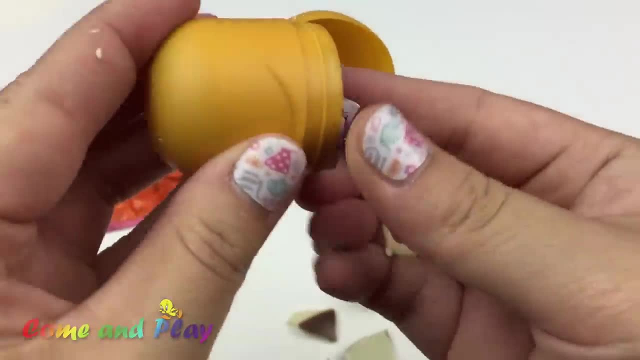 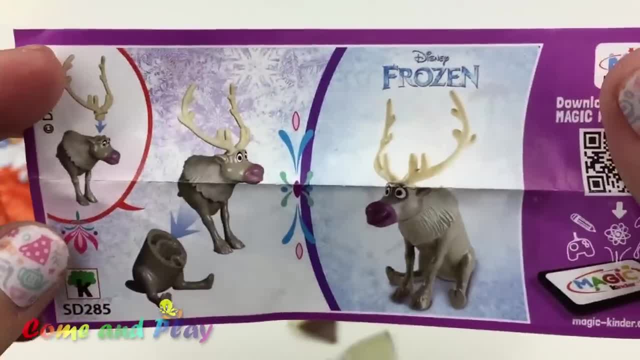 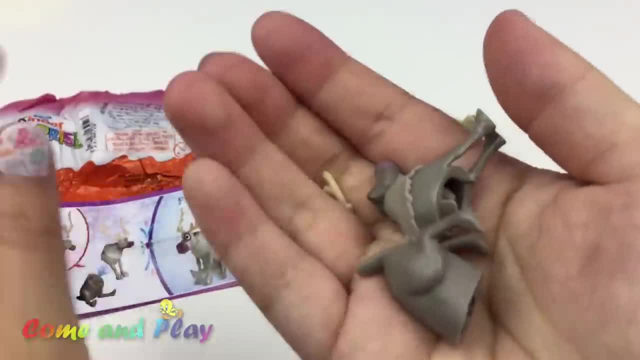 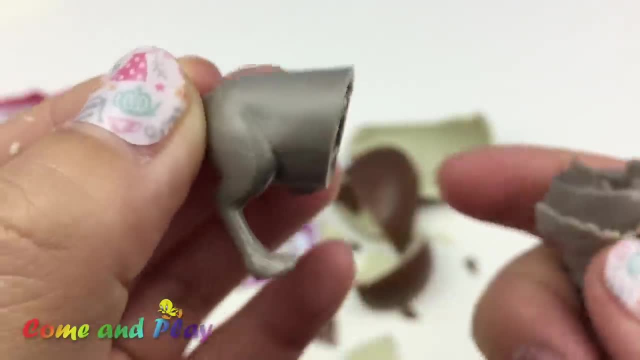 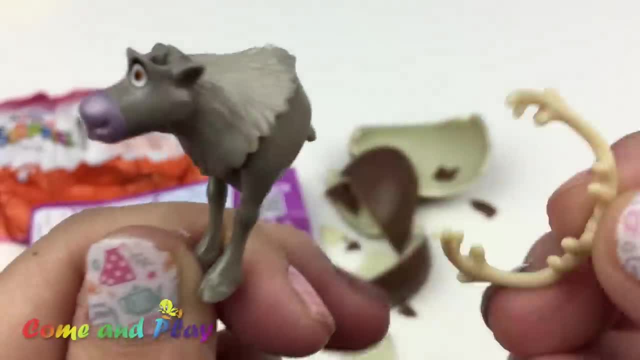 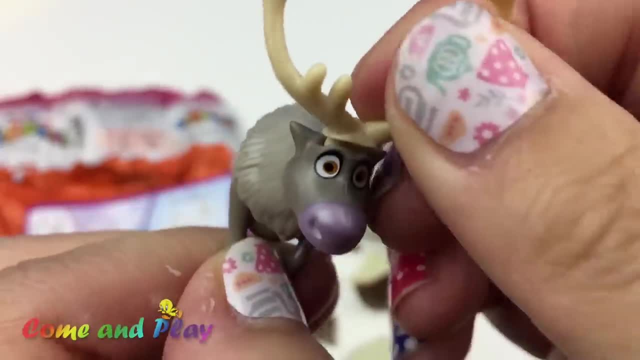 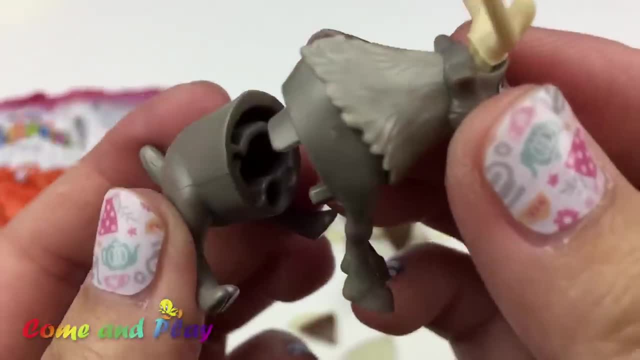 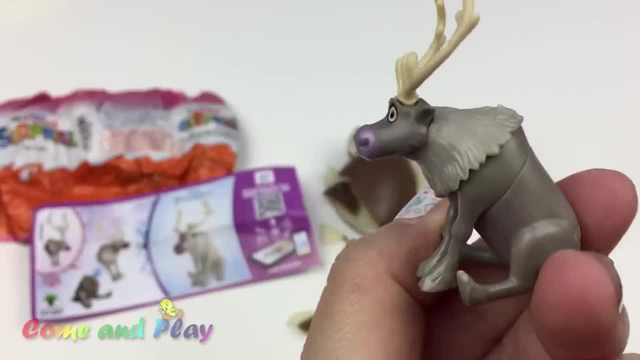